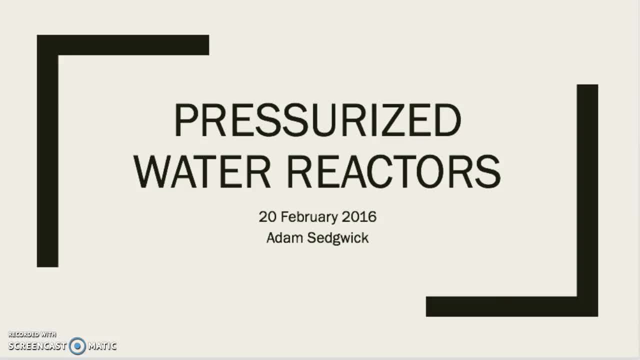 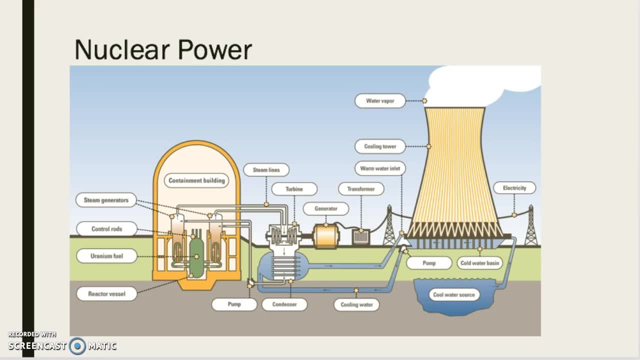 Hello, I am Adam Sedgwick and today I will be presenting a slide cast on pressurized water reactors. A pressurized water reactor is a type of nuclear reactor that creates nuclear power. Throughout the United States today, there are currently 100 nuclear power plants. 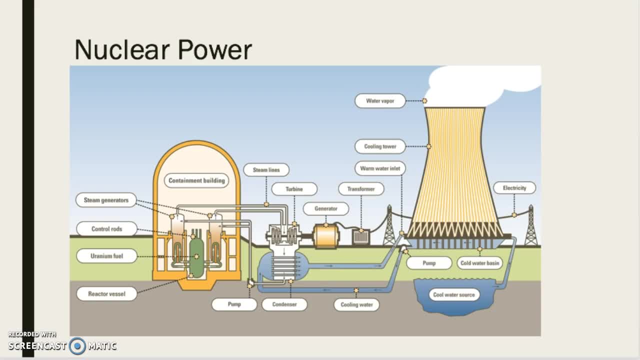 providing roughly 20% of the nation's electrical needs. That's a really big thing. That's a lot of electricity that these nuclear power plants are producing, And most of these power plants are pressurized water reactors. Also, the Navy submarines use nuclear power technology. 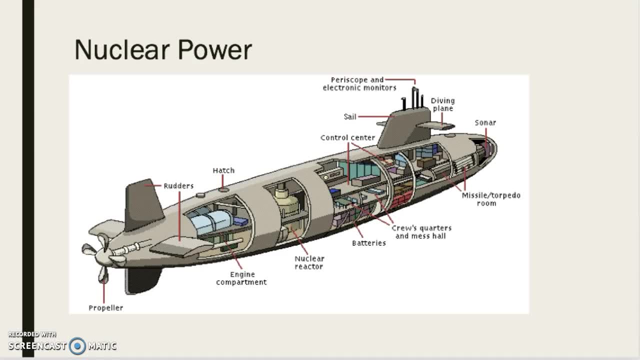 in the form of pressurized water reactors to operate and run. This could be said to be one of the primary foundations for nuclear power in the United States, starting with the submarines. Now let's look at the nuclear reactor and discuss how it works. It starts. 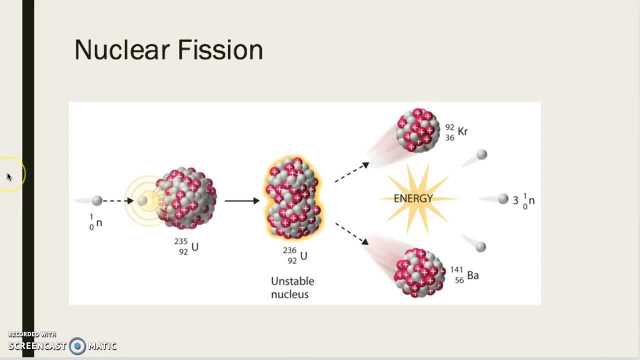 with a process called nuclear fission. A neutron is fired at a uranium-230 isotope atom and as it strikes the atom it creates a lot of intense energy and it creates a reaction. This nuclear reaction causes the uranium-230 isotope atom to split. 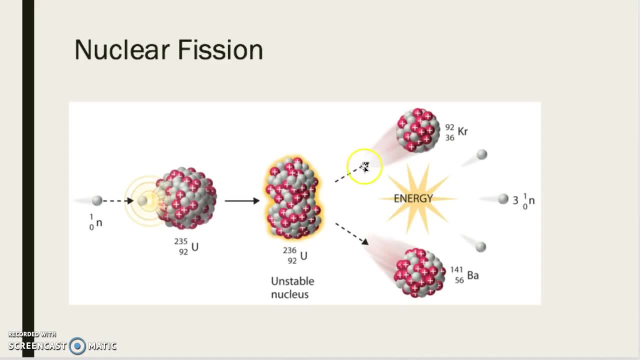 into two separate atoms, causing a large amount of energy to form and additional neutrons to split off from these atoms. These neutrons moving at high speeds hit other uranium-230 isotope atoms And this chain reaction begins and continues to create lots of energy and the chain reaction 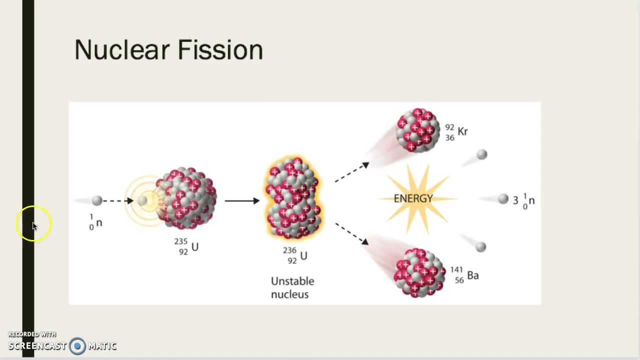 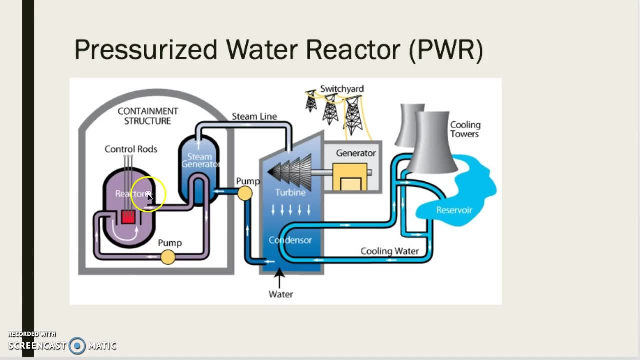 will go on for a long period of time if not stopped. So pressurized water reactors were developed in order to contain this reaction, in order to transform that energy into usable electrical energy. Quite simple, very effective, but the design is very important. So let's. 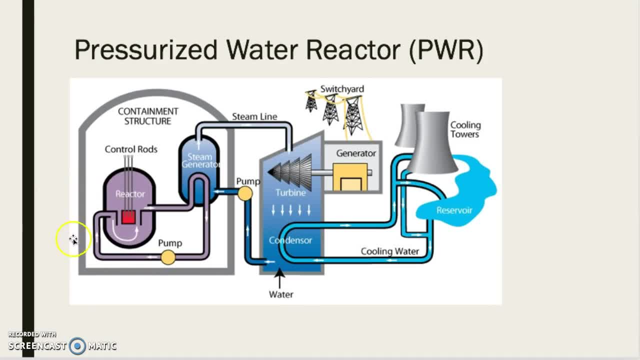 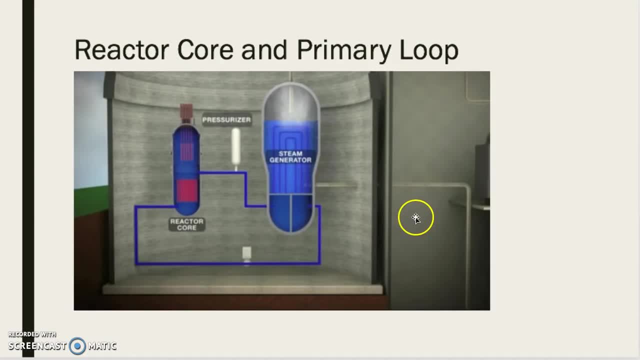 start with the first part, this primary loop where the reactor sits, the pump sits and additional components sit. So within this primary loop, water is heated by the nuclear reaction and it's pumped through the system. A pressurizer pressurizes the water up to 15.5 bar, which